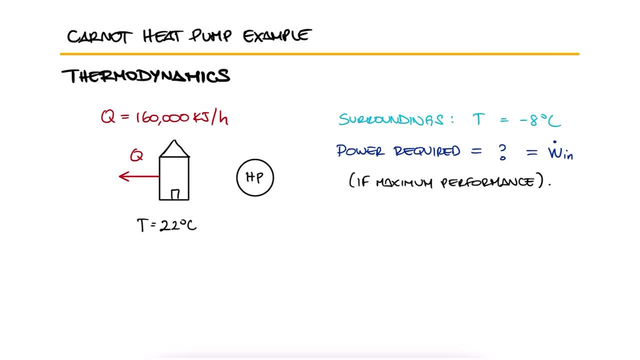 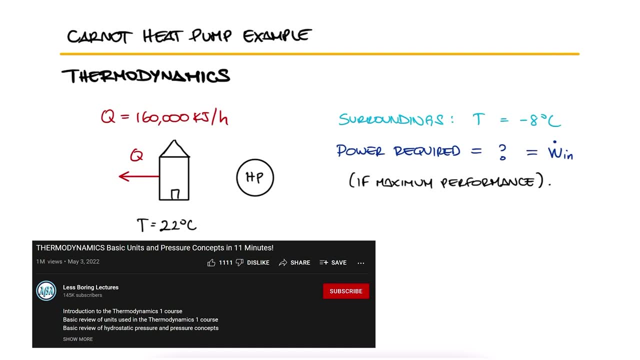 here and try solving this yourself before watching the solution. This is the first example for the Cournot Cycles and Reversible Processes main lecture. The link to that 12-minute lecture and all the other examples and lectures of the thermo course are found in the description. 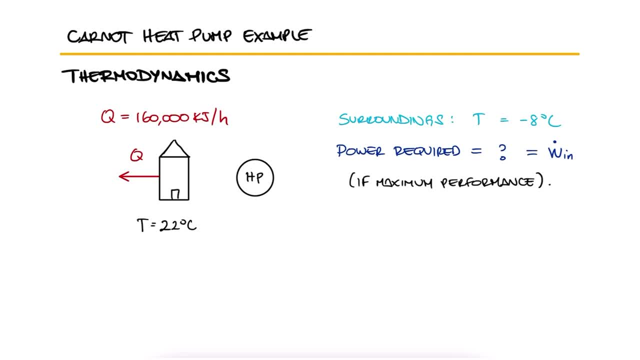 below, Similarly to the non-Carnot Cycle examples from the previous lecture, we begin by drawing the system. There's a heat pump that provides the house with heat, Since the house is at a higher temperature than the surroundings. the house is the high temperature reservoir. 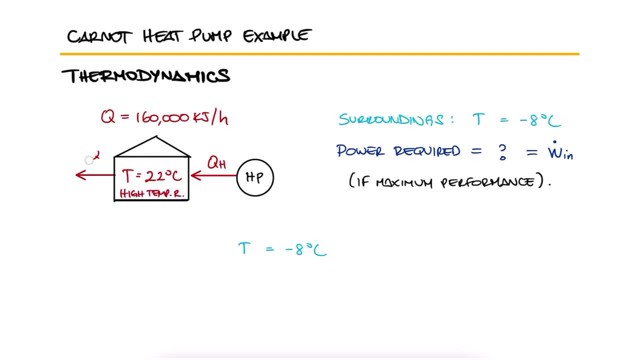 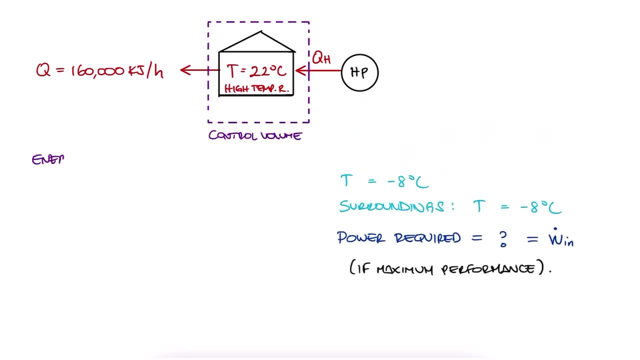 so we label this heat QH. The house itself is losing heat at the given rate. This means that if we draw a control volume around the house and for the house to remain at the constant temperature, the heat that comes in from the heat pump into the house has to. 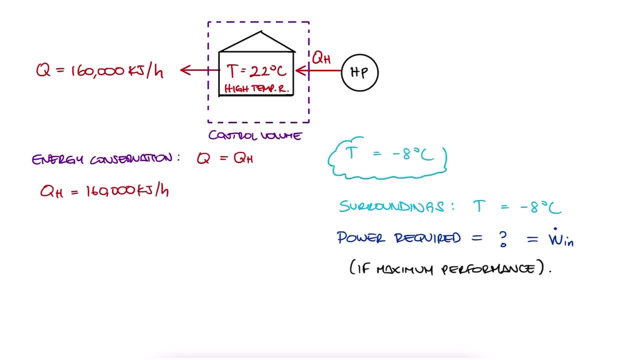 be equal to the heat rejected by the house And, additionally, there is heat being drawn from the low temperature surroundings QL and for this to work, we are adding a work rate N or power N To find this work, which is the difference between QH and QL, we need. 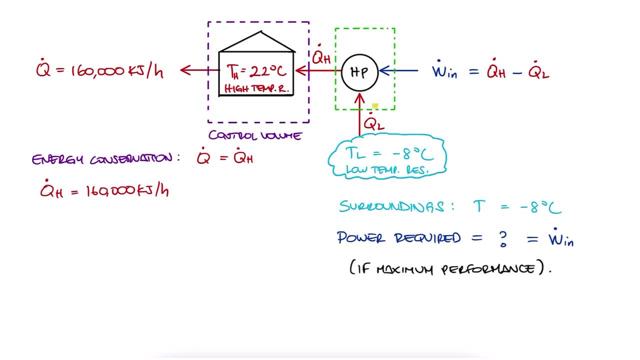 to find QL. So our goal is to find how much heat is being drawn from the exterior of the house. The maximum coefficient of QH is a positive temperature, which is equal to the heat that is coming in, which is the heat rejected by the house. So our goal is to find how much. 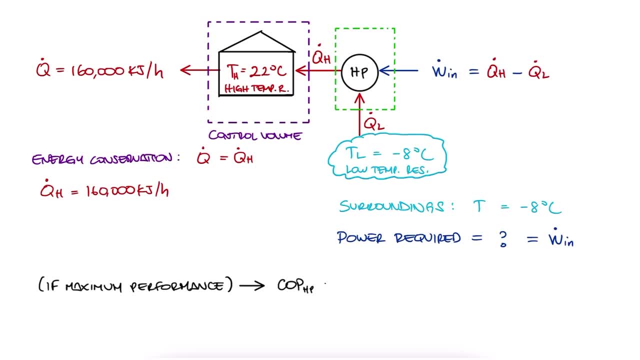 The coefficient of performance for this heat pump is when we substitute the heat variables QH over, QH minus QL with the temperatures, like it was explained in the main video. We substitute the temperature values in Kelvin, like explained in the lecture video, and find: 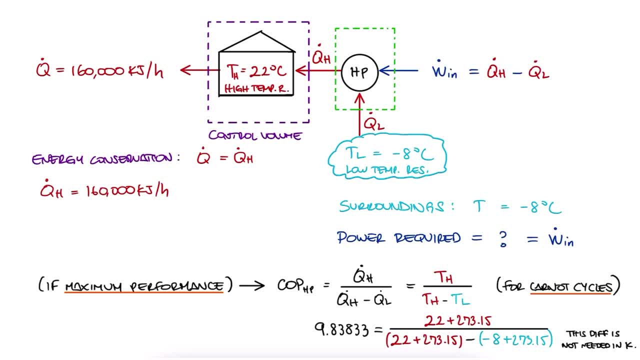 the coefficient of performance, And since it should still be the same in terms of heat variables, and we know that QH minus QL is the work that goes into the pump, we substitute QH and solve for W in dot, And that's it. 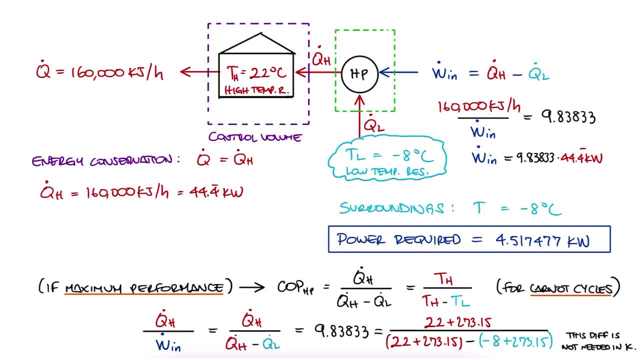 If you want to check out other examples for Carnot cycles and reversible processes, make sure to check out the links left down in the description below, where you'll also find the links to the other lectures of the Thermodynamics course, as well as other engineering courses. Thanks for watching.